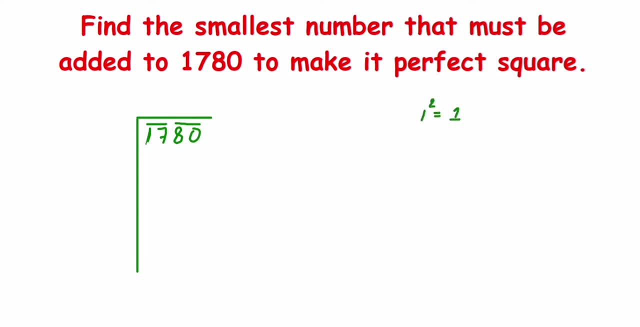 square near to 17.. So we know that 1 square is 1, 2 square is 4, 3 square is 9 and 4 square is 16, and next is like 5 square, which is nothing but 25.. So here I cannot take 25, I cannot take even 9, because 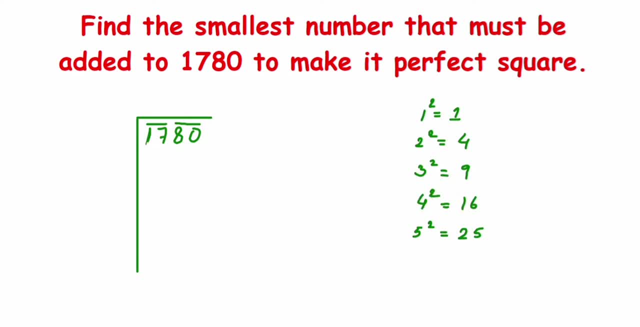 25 is greater, So I will go with 16 here. 4 square is 16.. So I will write down here: 4x4 or 4x4 is 16, and subtract it So we get the remainder 1.. Now I am going to drop 80 here, So I am going to drop the entire pair: 80,, not a single. 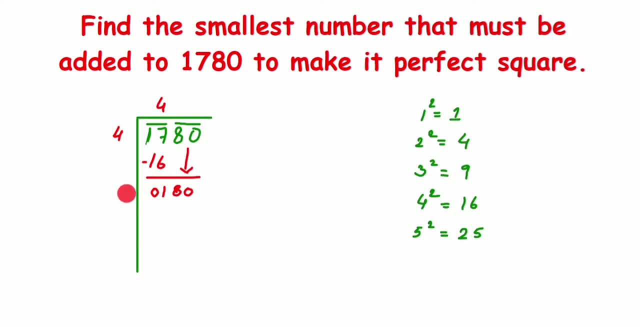 legit 8.. So now I got 180 here. Now to find this, I have to find the divisor and how to do that. Take the double of the question. So here the question is 4.. Double of 4 is that is 4, twos are 8.. So I am going to write down 8 here, But that is only a one single. 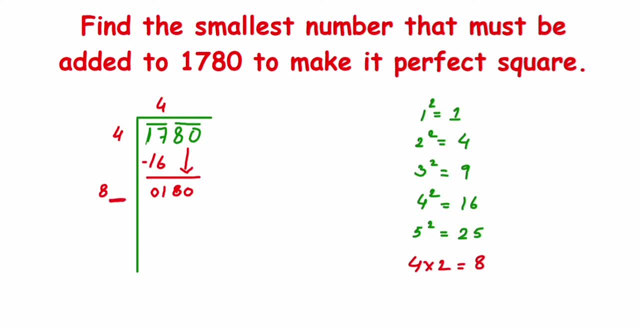 digit. I need to find out a number in the ones place, or the unit digit And remember the unit digit. and the new question has to be same here. This: both number has to be same. So for that we are going to take a number. For example, I will write down 81 multiplied by 1, which is going to give us 81 again. 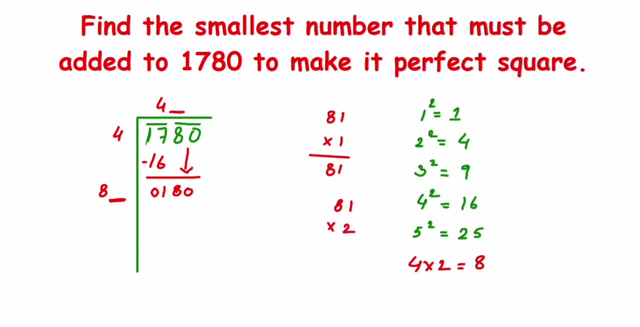 here And next 81 multiplied by 2.. This I cannot take because 1 and 2 are different numbers. right, 2 is a question, 1 is in ones place, So they has to be same. Now I got 81. ones are 81. So, but still small. I will go with next number. 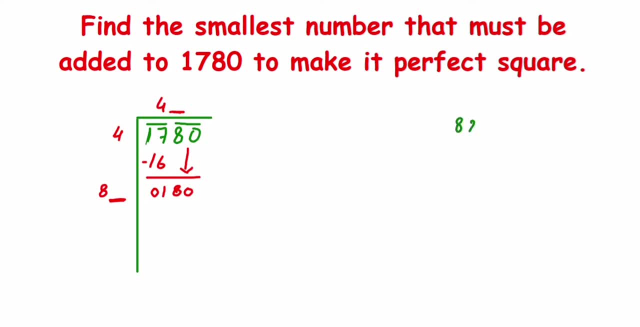 So I will write down here: 82 multiplied by 2.. So this is going to give me 164.. It's still small. Let us try with 3.. So 83 multiplied by 3 is 249.. This number is greater, So I will go with 164.. 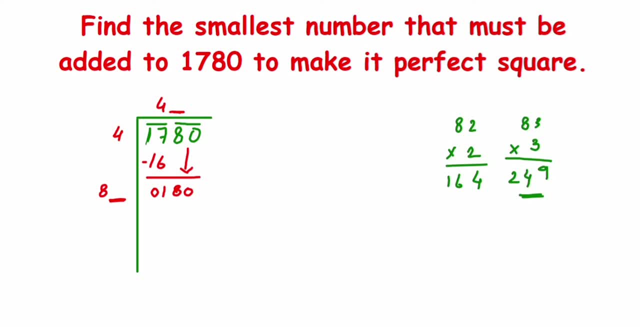 That is 82, twos are. So I will write down here: 82 multiplied by 2. We are going to give me 164. So we will just subtract it. So once you subtract here, you will get the remainder as 16.. 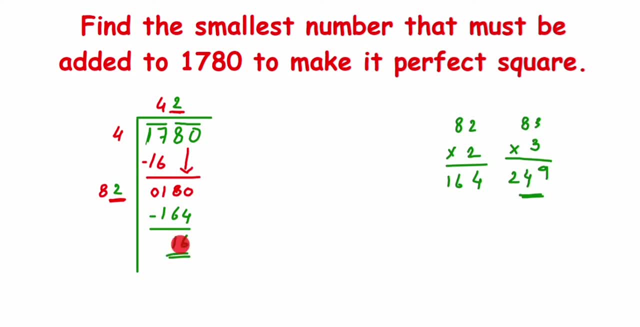 Now. so we got the remainder 16.. This means that this given number is not a perfect square. So what will be the next perfect square? Here? we got the question: 42, right, It means if the number is perfect square, the answer would have been a 42.. So this means that the 42 square is less than 1780.. 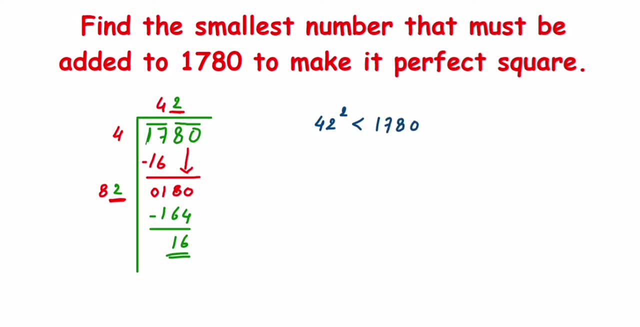 Remember, I have taken 42 square because the quotient- what we got here- is normally a square root Now, so 42 square is a perfect square. The next perfect square will be 43 square, So 42 square is less than 1780.. Next perfect square will be 43 square, So I am not going to open 42. I will just write. 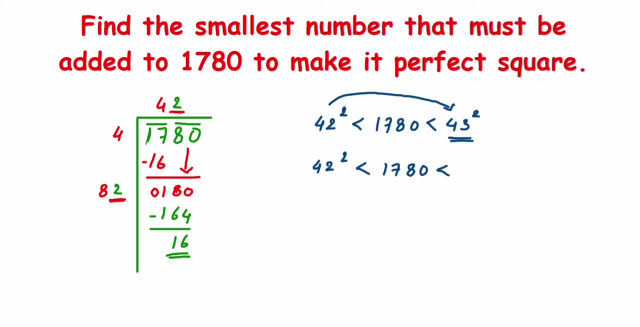 42 square is less than 1780, which is again less than 43 square, which is nothing but 1849.. So 1849 is a perfect square. So we have to find out how much we should add to 1780 to get 1849.. 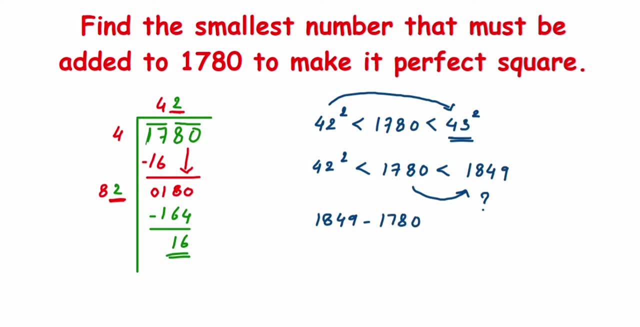 So just simply subtract it. So 1849 minus 1780.. So when you subtract it, we will get 69 as an answer. So the smallest number which has to be 1849.. So the smallest number which has to be 1849.. So the smallest number which has to be 1849. 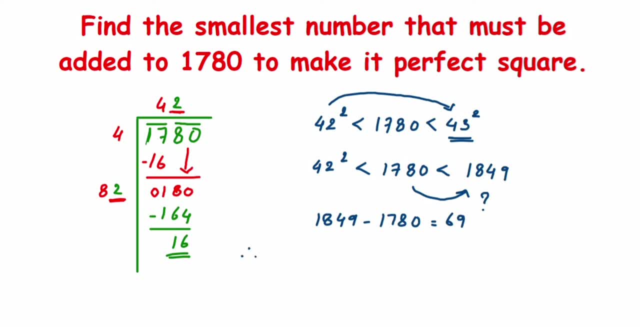 added will be 69.. If I add the 69, I'll get the answer. So 69 I gonna add to the given number. so we can just conclude first here. therefore, 69 is the smallest number to be added, And when I add this, let us add this number. So once I add this, 1849, now the number 4 will be sowie 89. 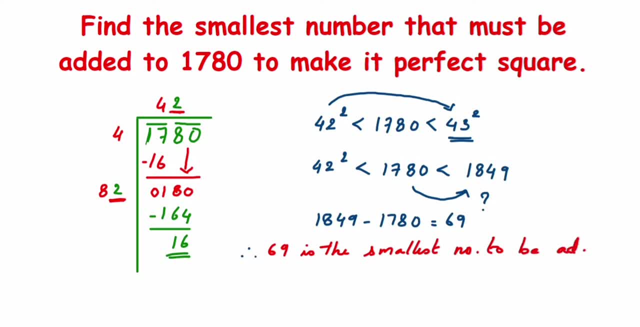 So when I add this to the given number, therefore 69 is the smallest number to be added, And when I add this, So when I add this, let us add this number. So once I have this 1849, I will get sorry- 1780 plus 69, we're gonna give us 1849, and 1849 is a perfect square. when you find out a. 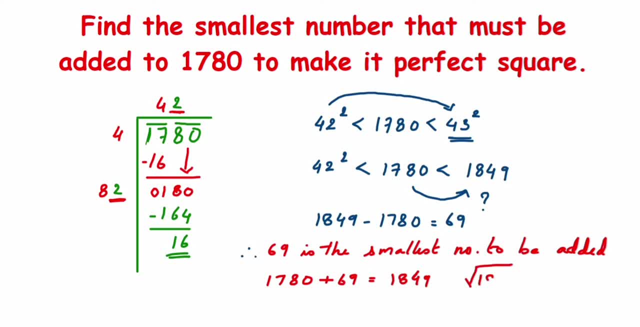 square root of 1849. that is, square root of 1849. you will get the answer: 43, that's it. so this is how you have to find out the answer. whatever questions you got it. that is 42, we got here. you take the next number and take the square of it. that's it. i hope it's clear.